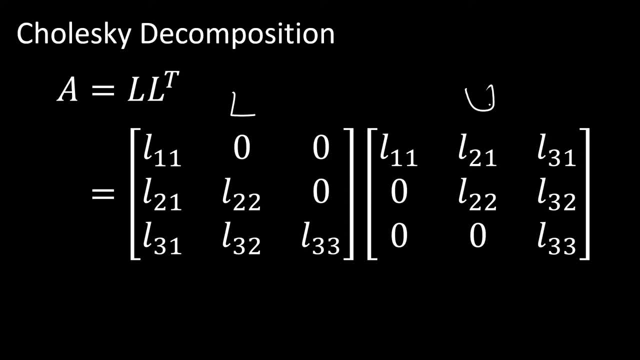 have a lower triangular matrix and then an upper triangular matrix. It's just that our upper triangular matrix in this case is just equivalent to our lower triangular matrix transposed. This is the key benefit of the Cholesky decomposition. We only need to keep track. 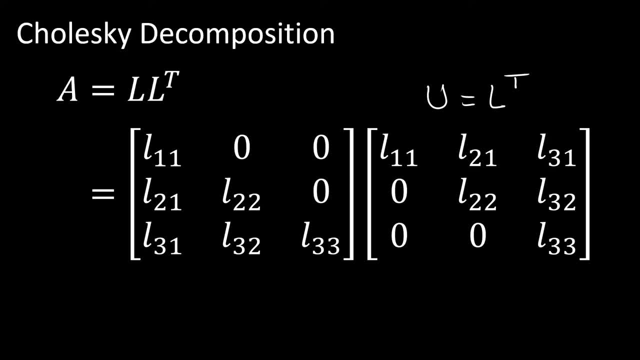 of the values of one matrix, since we can just then transpose it and then write: multiply that lower triangular matrix by that triangle. This should be seen as an important property of an that's close. To open up our questionnaire first, you simply plug in this output: Bernoulli matrix dot analysis. 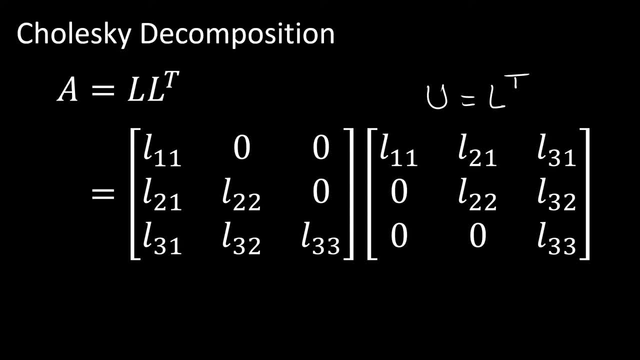 In this case there is no useful relationship between this material and the Chiolesky program. here transpose and then get back to our A matrix. But all higher level matrix decompositions have initial conditions that must be satisfied for us to be able to do that matrix decomposition. 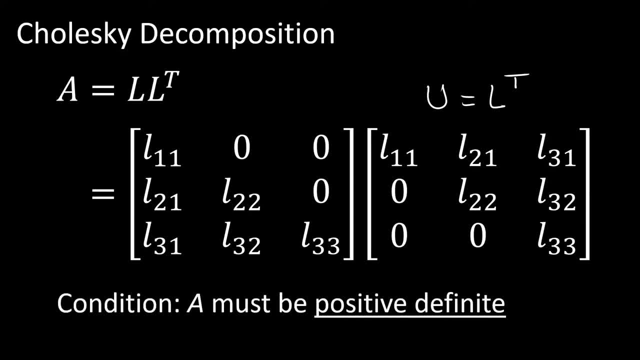 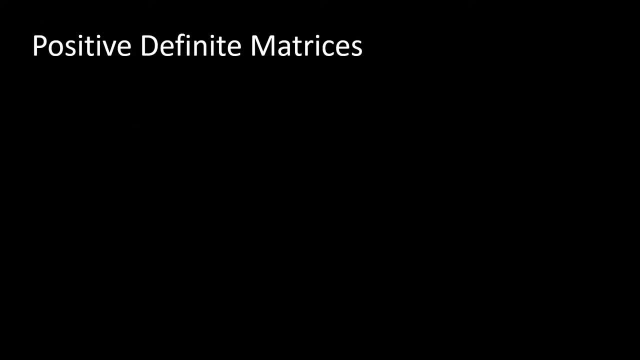 For the Cholesky decomposition. that initial condition is that our A matrix must be what is called positive definite. So what is a positive definite matrix? Well, a positive definite matrix is much more of a pure linear algebra topic, not so much a computational. 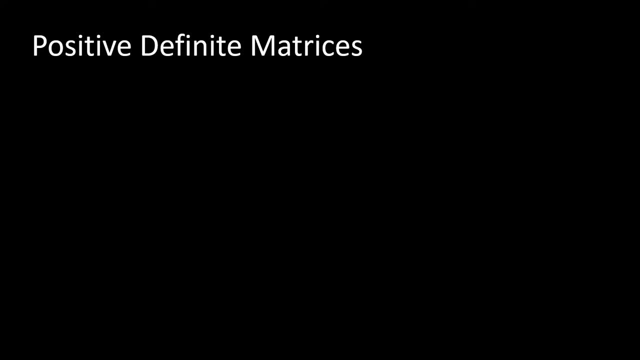 linear algebra topic, so I'm not going to go into too much depth with this. I'll leave a few links in the description down below where you will be able to find more information on positive definite matrices from a pure linear algebra standpoint. I instead am just 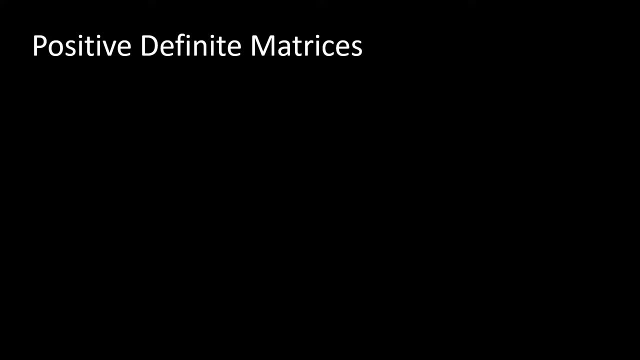 going to quickly go through and review some of the key concepts of a positive definite matrix. First, all the eigenvalues of a positive definite matrix must be positive. All the pivots must also be positive, All the subdeterminants of the matrix must also be positive And, generally speaking, 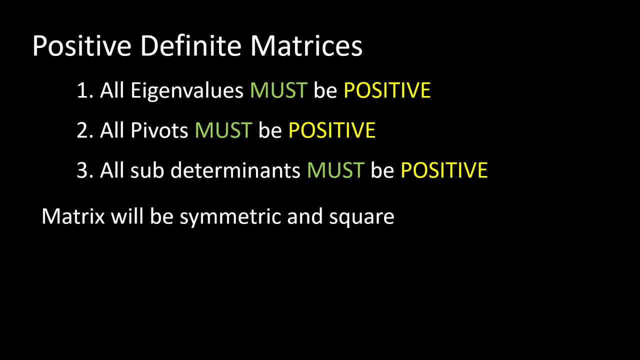 the matrix will be symmetric and square. Again, that's a generalization and for this particular video, we're only going to be considering symmetric and square matrices, And that basically just means that any off-diagonal values- so i not equal to j- will give us that a i j is. 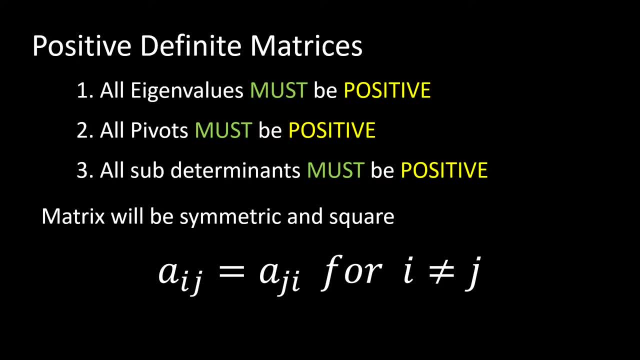 equal to a, j, i, if we're using i and j as our indices. Again, there will be links in the description down below for more resources where you can find out more about positive definite matrices. So we're going to jump right into the code on how we can actually 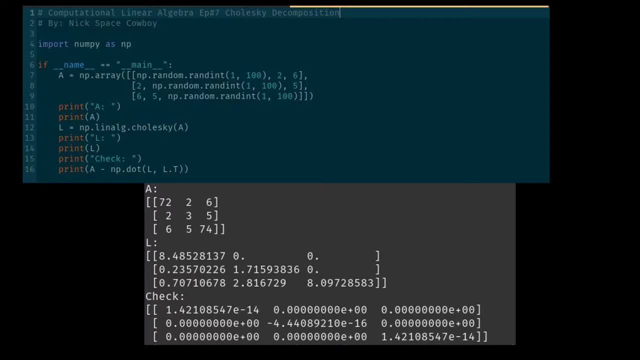 perform a Cholesky decomposition, because there are very quick ways of doing a Cholesky decomposition in both Python and Octave, and you can see we're starting off with Python. Per usual. all of this code can be found on Pythoncom. 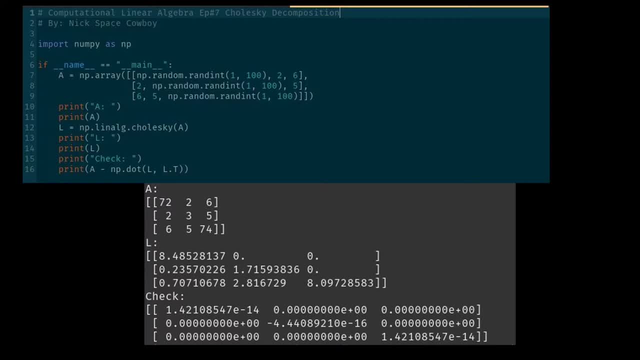 So you can find some of this code on my GitHub and Gitlab pages linked in the description down below. so I will encourage you to check that out and fork the repo and start playing with all of this code. You can see that this is really just some simple driver code, but you can see in line. 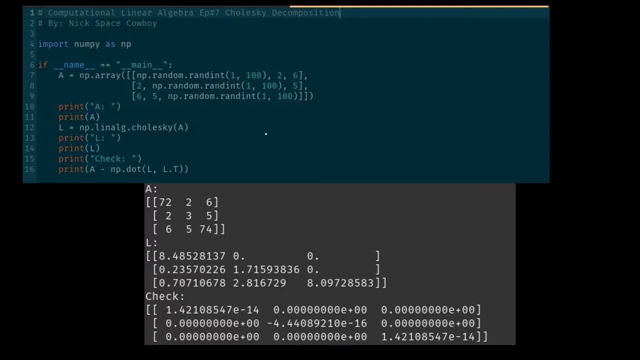 12. we are using the numpylinalgecholesky function right here, which is going to do the entire decomposition for us. You can see that I have a 3x3 positive definite matrix where we're generating random values along the diagonals right here, and then you can. 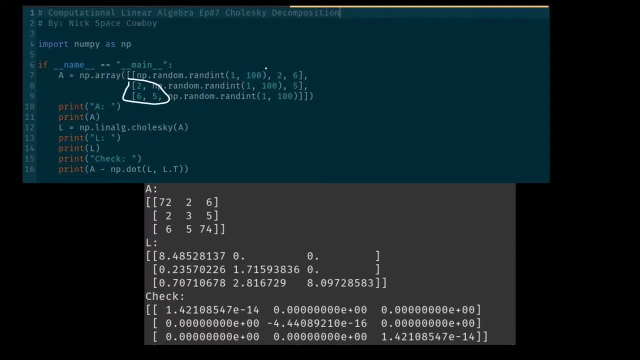 on the anywhere off the diagonal, we have symmetric values. Then what we're doing is we're just going to output that to the terminal window and, as a check, this time we're subtracting a minus l right multiplied by l transpose, and you can see that in the terminal right. here we have this standard. 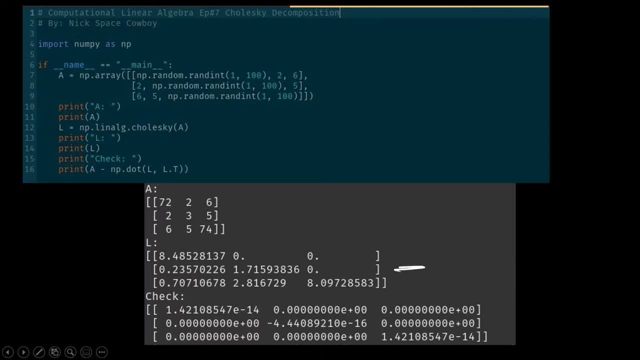 output. this is our, our one matrix, because, again, this is the advantage of the Cholesky decomposition- we only need to keep track of one matrix. This matrix is generally referred to as the Cholesky factor, by the way, and you can see that when we check everything out, everything is pretty much. 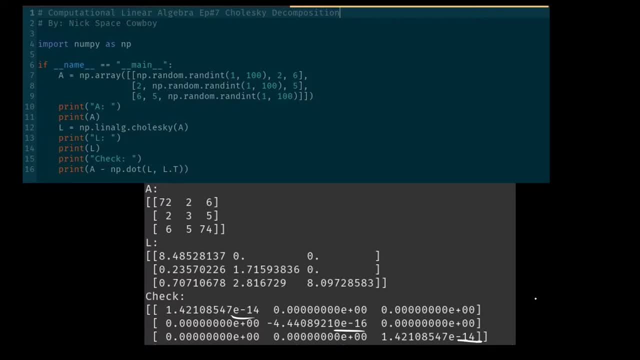 zero with, except for these diagonal values which we can, which are very small in value and we can attribute to floating point arithmetic error. so we can just approximate those to be zero and everything checks out. Moving on to the octave code, you can see that we're doing something very 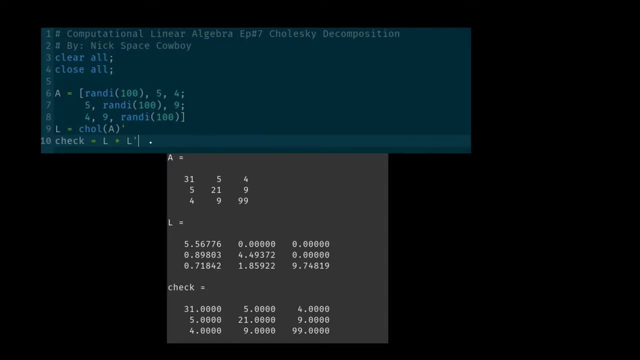 similar. we're doing a different three by three matrix. but you can see it's even simpler. we have in line nine, this Scholl function that we're passing our matrix into. Bear in mind that octave uses the Cholesky factor or the return matrix as the upper triangular matrix. so in turn a would equal l, transpose l in octave, so we're. 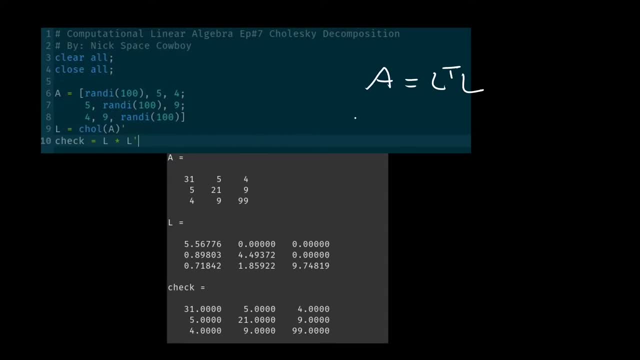 just transposing it with the single rotation mark right there. Then we can go ahead and check everything out with l by l transpose, we're not subtracting anything off- and you can see and just spot check everything that it all works out. and again, here is our Cholesky factor or our l. 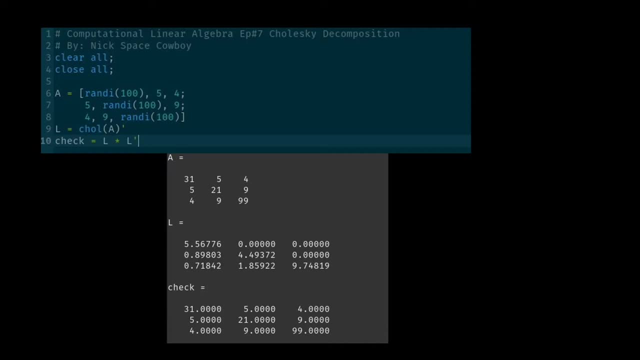 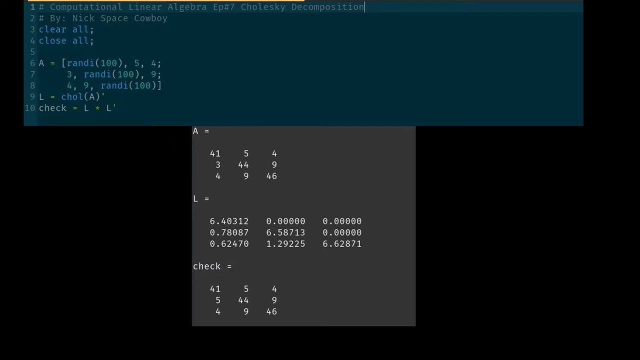 matrix that we are returning Again, the key advantage being that we only need to keep track of one matrix. But do note that there is something a bit peculiar with both of these functions: If we change one value in our square symmetric matrix to a different value, so this value should. 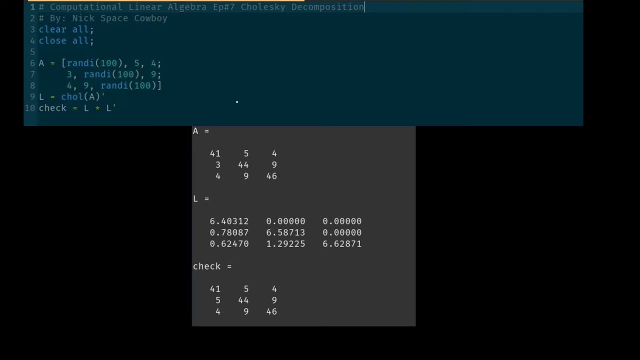 change to a three, you can see that the code still runs, even though it's not symmetric, and that's because the matrix here passes the check on the back end for positive definiteness. You can see that we still obtain a Cholesky factor, but we return back a matrix that is symmetric, and this 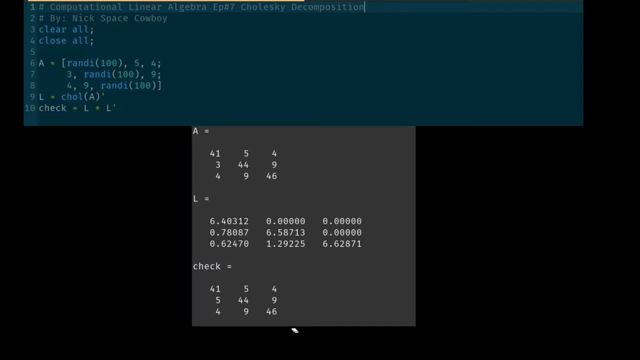 is a key flaw with the basic algorithm that is used to check for positive definiteness. We're going to go over that in a moment, but just bear in mind that this is a significant flaw And checking if a matrix is positive definite or not is still a very difficult and very advanced. 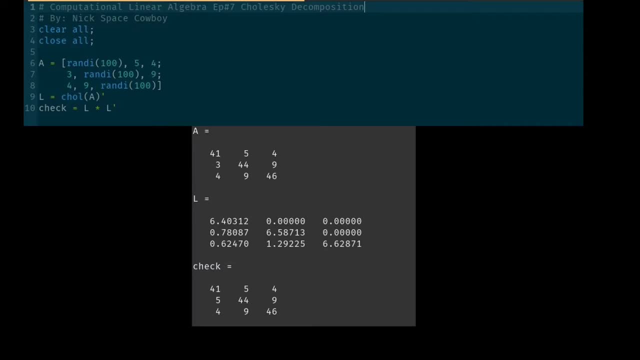 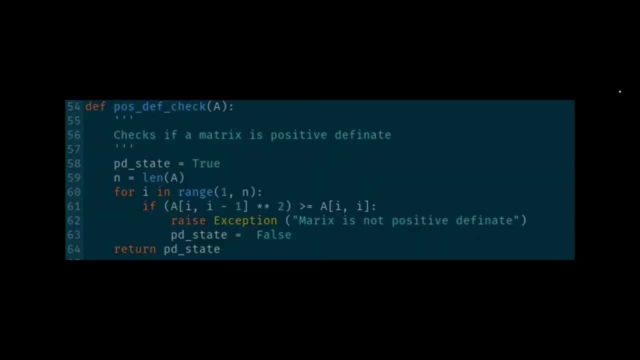 topic in linear algebra. That comes largely in part that identifying or obtaining eigenvalues and pivots and even calculating sub determinants is still a little bit tricky and very computationally intensive. So here in our lin-alge package we're going to take a look and take a stab at the back. 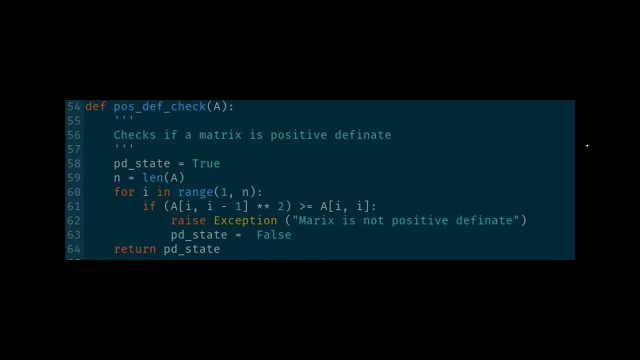 end procedure of how we actually check if a matrix is positive, definite or not. So here in our lin-alge package we're going to take a look and take a stab at the back end procedure of how we actually check if a matrix is positive, definite. So if you go into the lin-alge directory in the GitHub repo under the 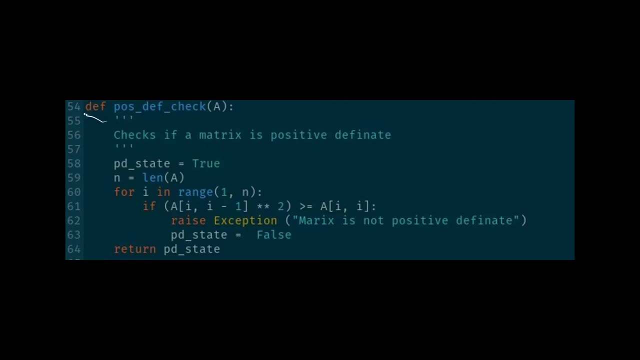 seventh episode folder. you will see in line 54 we've defined this new function called positive check, which checks if a matrix is positive definite. That's why we're passing in our a matrix. We can just do a simple Boolean expression right here where our positive definite. 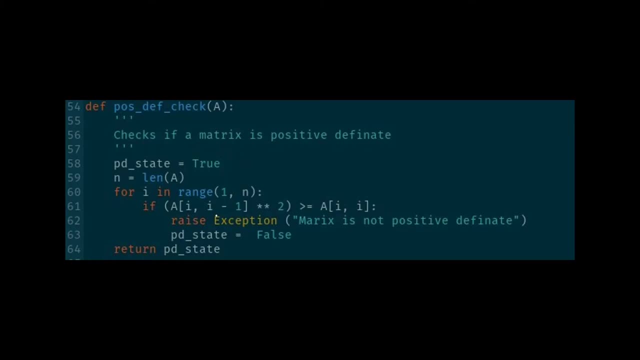 state is default, set to true, and if any of the values just before the off diet, just on the lower off diagonal squared, are greater than or equal to the values on the diagonal, then we will raise an exception that the matrix is not positive, definite and change our state to false, which then we are returning right here To give a good example of this: 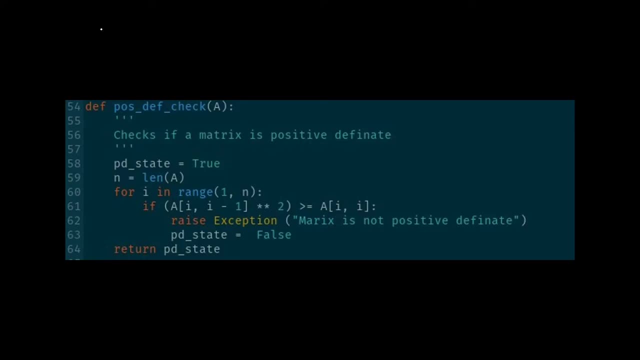 and where this flaw really takes place. let's say that we have an, a matrix, and we have one, two, three along the diagonal. We're not going to worry about anything above the diagonal right now. just assume that it's filled in with random values. and let's say that we have four, five and 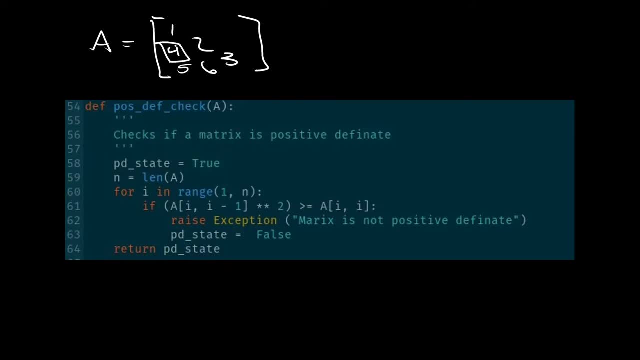 six right here. These values are the ones that are going to. these boxed values are the ones that are going to be squared and compared to their counterpart in the algorithm, just to the right in the matrix. and this is going to continue to go on for larger sized matrix matrices, and that's a. 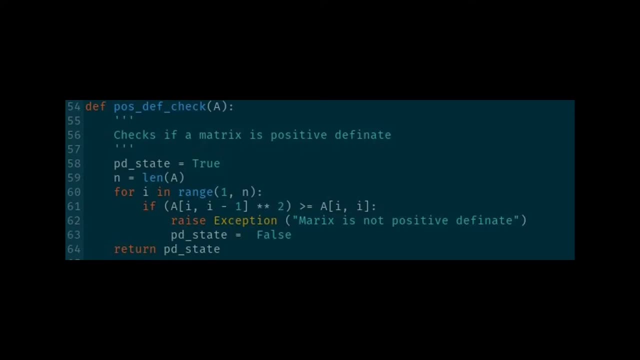 key flaw in this, in this is that it allows us to check. if a matrix is positive, Definite. but if you don't put in something that's symmetric, it will give you back something that is symmetric. when going through and checking everything out, We can really begin to see. 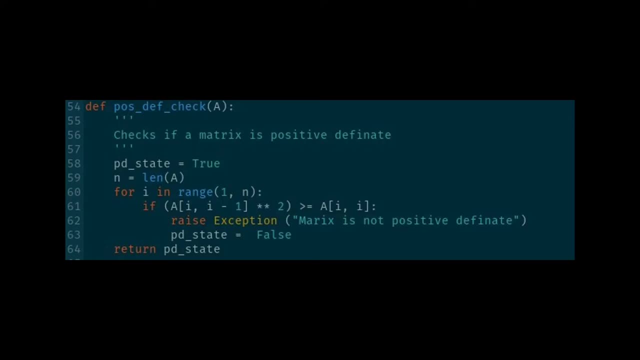 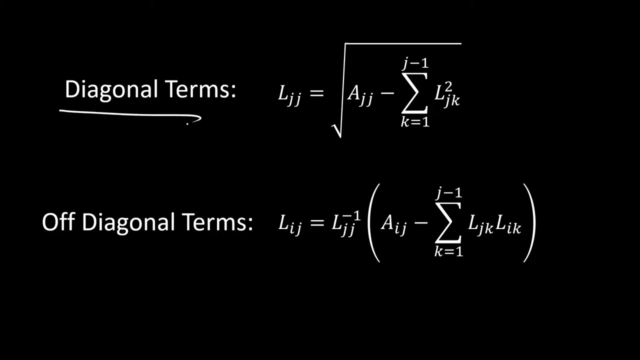 where these problems lie. when we take a look at the equations that we're going to use to compute the Cholesky decomposition. Here you can see we have an equation for computing our diagonal terms and our off diagonal terms. In both of these equations you can see that we are reliant. 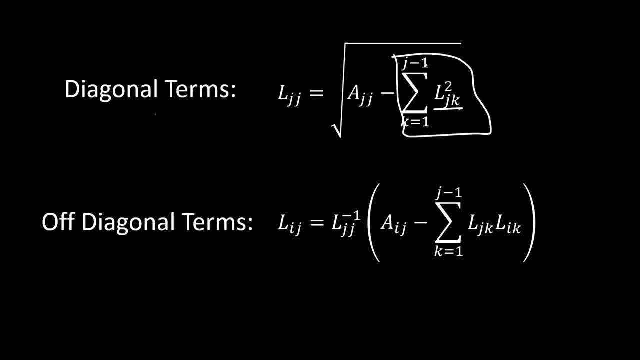 on this sum term right here. We're going to use this sum term to compute the diagonal terms here where there is a dependence on other values within our lower triangular matrix that we are generating right here. You can see all of them right here. This makes things a little bit tricky. 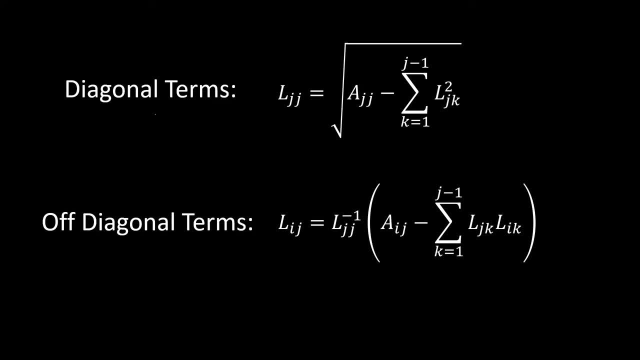 and is why it will return back a symmetric matrix that is not equivalent to the original matrix that you put into the function of these two equations for the diagonals and the off diagonals. This poses an interesting little bit of complexity When we are coding it up. so let's take a look at how I've coded that up in the back end in Python. 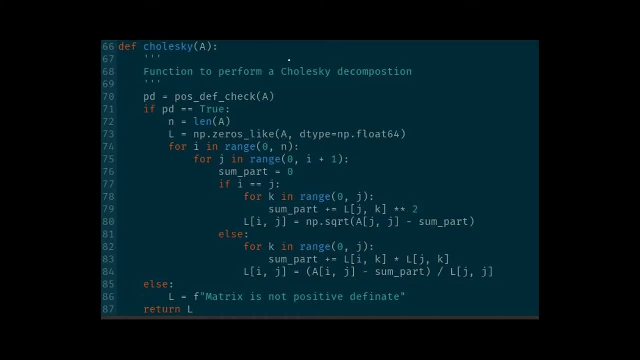 In the same lin-alg package you will go and see just below our positive definite check, in line 66 I've defined a new function called Cholesky where we're going to pass in our a matrix. Then you can see we are calling our positive definite check function and we're setting that. 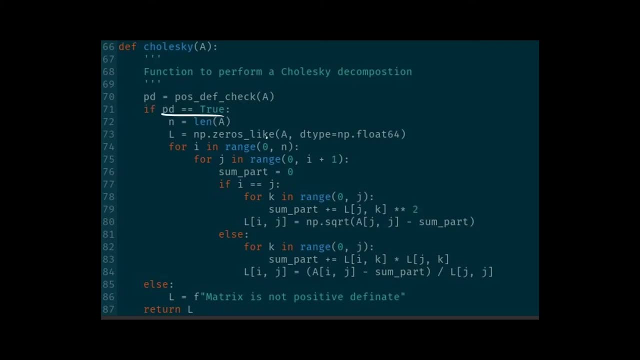 state equal to the variable pd. If our positive definite check comes back as true, then we're all good to go. If it doesn't, we will see that we will see that exception be raised from the positive definite check function. but I've also added in this extra little line right here this else statement, so that 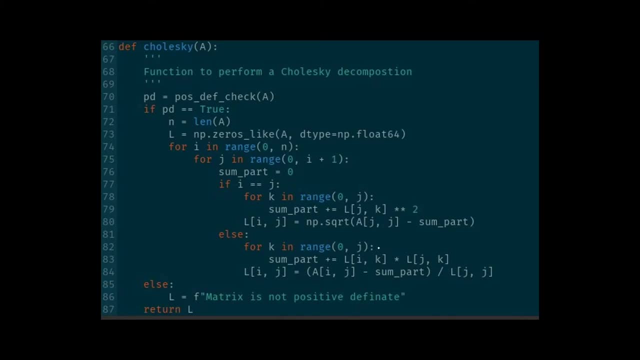 just in case you know, whatever the heck might happen goes wrong, we will also know that the matrix is not positive, definite, so we can't perform the Cholesky decomposition. Then we just need to worry about one particular matrix. Again, this is the Cholesky factor. and then we have two loops right here, two, four loops to help us. 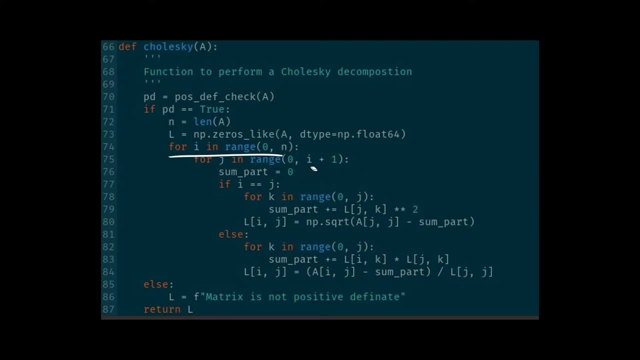 keep track of our indices. Then you can see we have an if else statement right here. this if statement is for the diagonal equation right up here on top and the else statement right here is for the off diagonal equation. Then you can see we have these two loops right in here. these loops are there to help us keep track of. 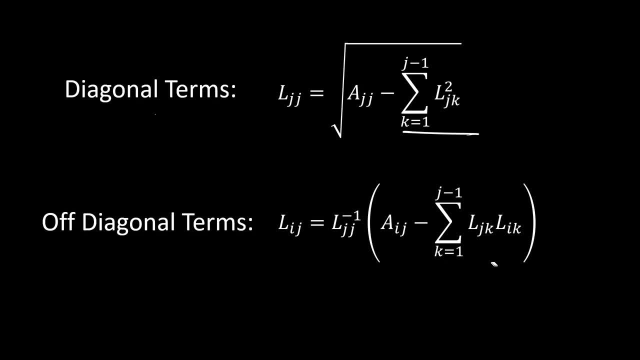 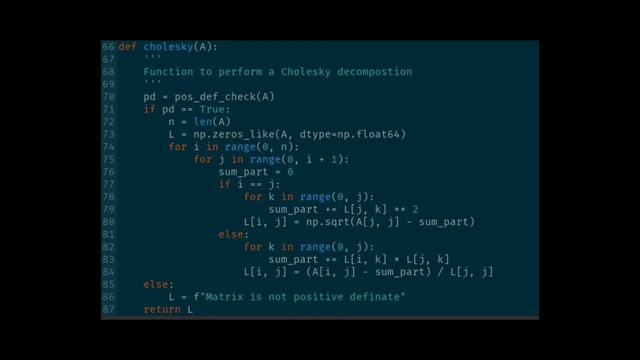 these summations in the two equations and then, per usual, we're just returning our Cholesky factor or this message, if we need that message for the driver code, which this one is the shul dot p y, file in the repository. For the driver code, which this one is the shul dot p y, file in the repository: 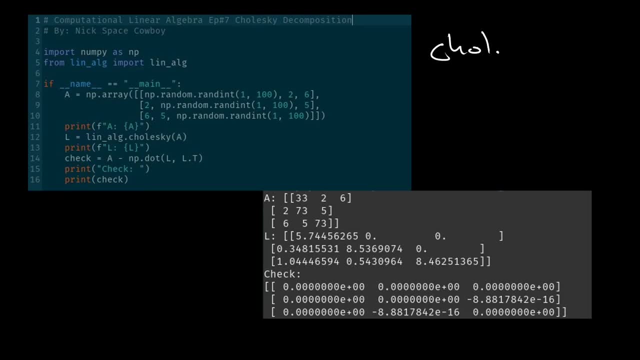 For the driver code, which this one is the shul dot p y file in the repository. This is just simple driver code. it's not very different from before. but instead of calling the Cholesky function in NumPy- we're from Linalge, we're importing our Linalge package and then we are calling that particular Cholesky function. 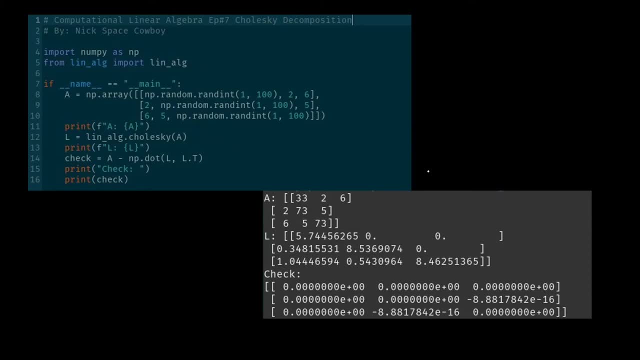 Then we're doing the same exact checks as before, where we are going to be subtracting our A matrix by L, by L transpose. So you can see, here is our matrix. We have our Cholesky factor, Our A matrix, Our matrix. 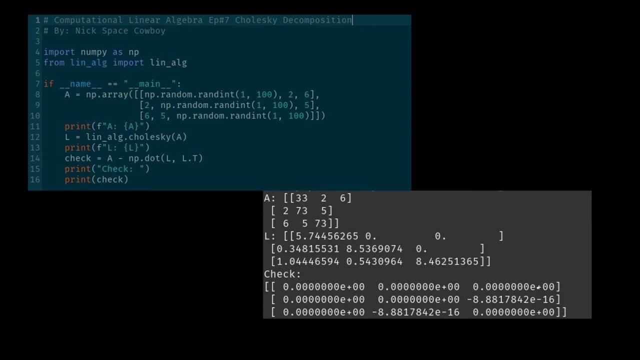